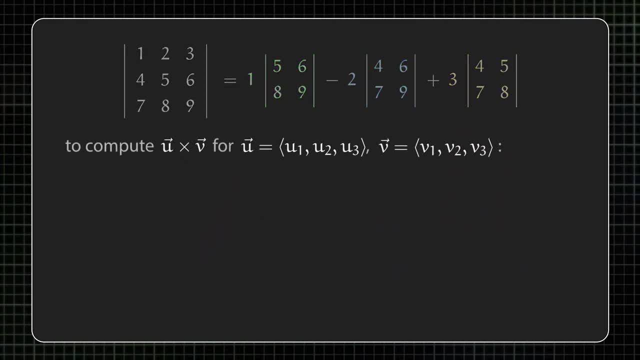 Now to use this to compute the cross product of two vectors, we build a 3x3 matrix where the first row consists of the standard unit vectors i, j and k and the second and third rows are the vectors that we want to cross. 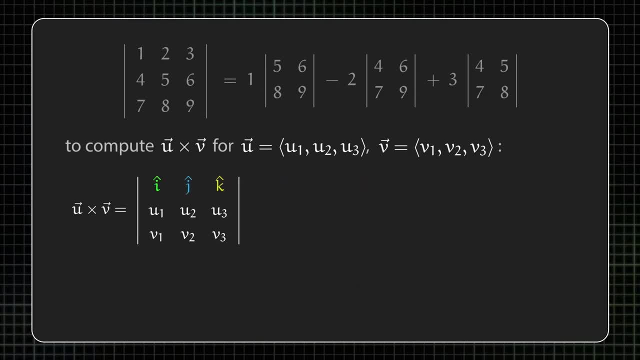 Taking the determinant of this matrix by expanding along the top row gives us an expression that looks like this: And if we remember that i, j and k are just stand-ins for the unit vectors, then the expression we end up with is the same. 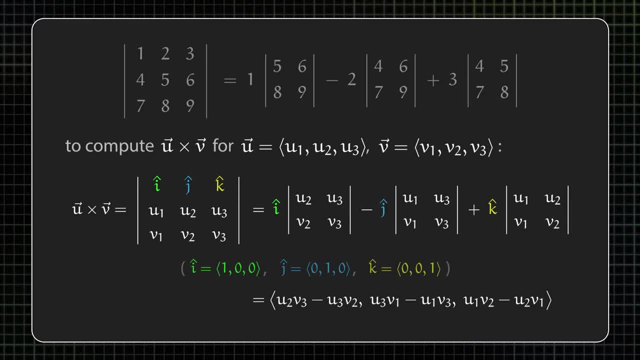 as the formula for the cross product that I showed you at the beginning of the video. So instead of remembering the formula, you can just remember the algorithm to compute 3x3 determinants. I think that's a little bit easier, but your preference may vary. 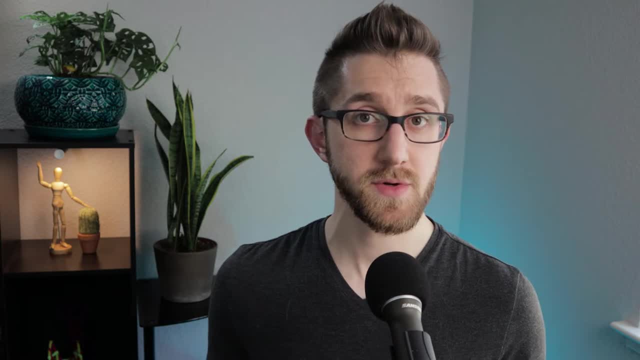 So that's how we compute cross products. But before we get into the written rubric and the return result, this is just an sucker tank. We'reフ0x1s- We know the formula for half a color in. There's a table of non-legal, easier formulas in that table. So before we get into the review of the 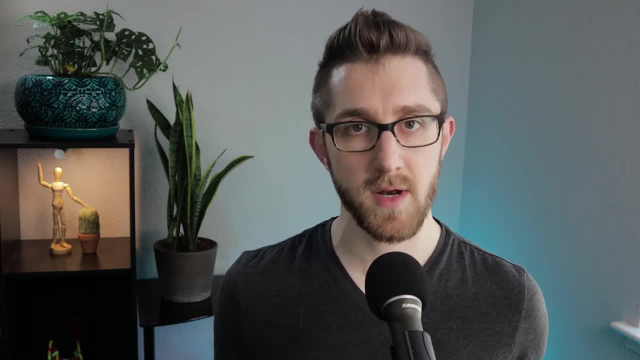 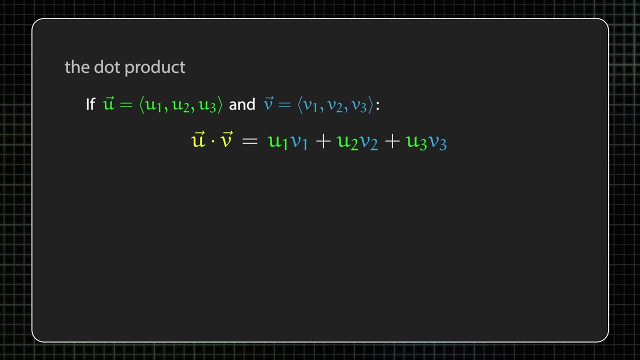 reasons behind why they're perpendicular. I should say a little bit about what it means for two vectors to be perpendicular. Enter the dot product. The dot product is another way to combine two three-dimensional vectors together, except it's fundamentally different from the cross product in that its output is 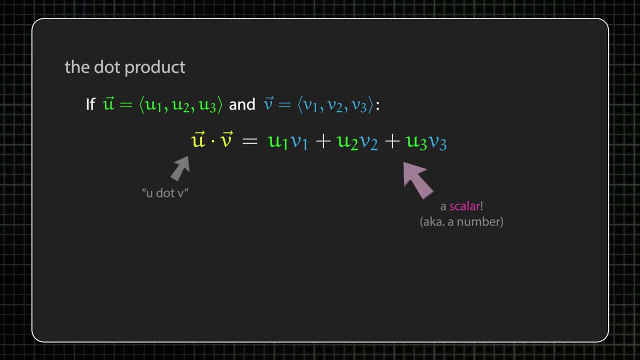 a scalar, or in other words it's just a number. But the dot product has its own host of useful geometric applications. In particular, the dot product of two vectors is zero exactly when those two vectors are perpendicular. So if two vectors form a right angle when you put their tails together, then their dot 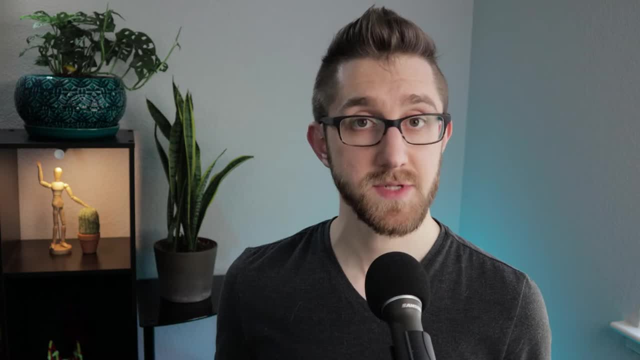 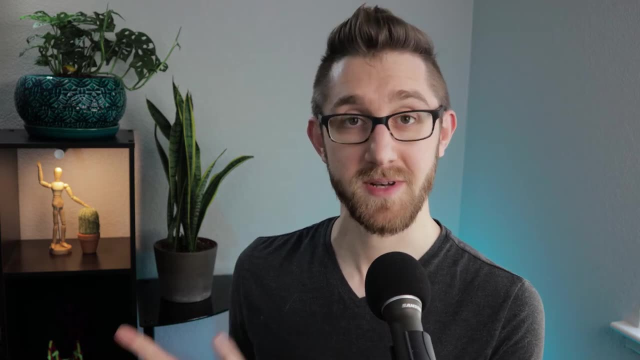 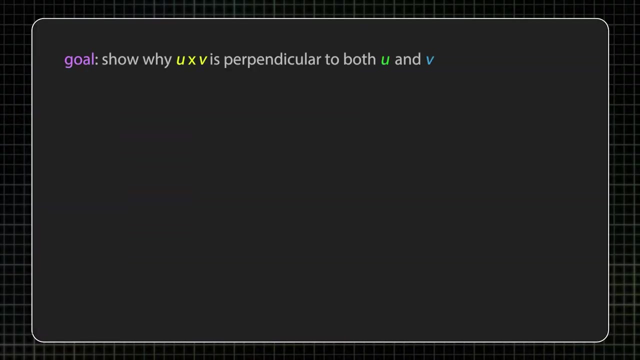 product is zero and vice versa. Okay, so we know about cross products and how to compute them using determinants, and we know about dot products and the relationship between dot products and perpendicular-ness. Let's put those things together. So our original goal was to show why the cross product of u and v 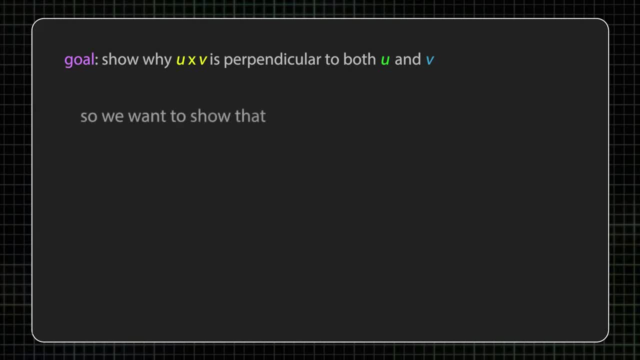 is perpendicular to both u and v. From what we've discussed about the dot product, this is equivalent to saying that u- dot u cross v and v- dot u cross v- are both zero. Let's just focus on one of those two statements. It's worth noting that we could just directly compute this.